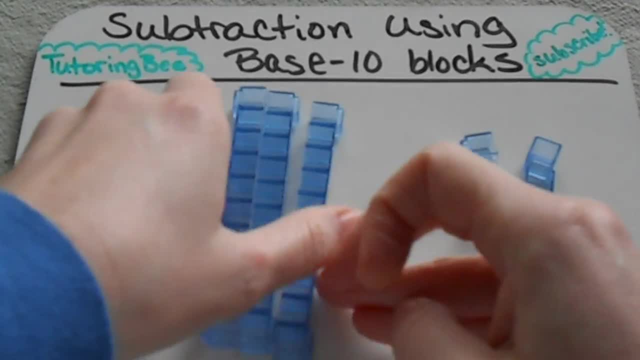 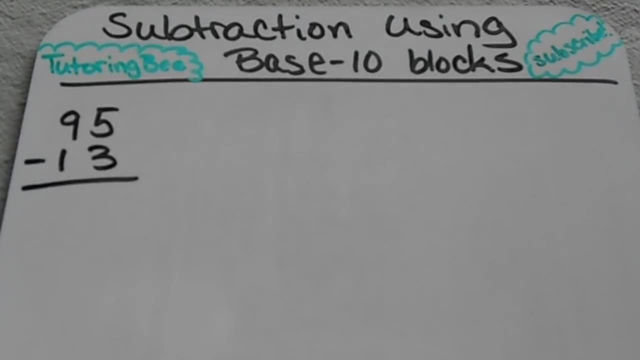 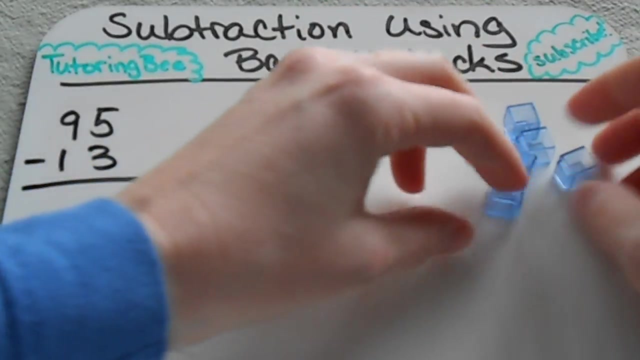 hundreds place, which are called flats, And I'm going to show you how to use the manipulatives and how you can draw them on your own if you don't have the manipulatives handy. So I have a pretty basic subtraction problem here: 95 minus 13.. So I'm just going to set up that top number, 95, and I do that by putting in 5 ones, and then I'll need 9 tens to set that up. 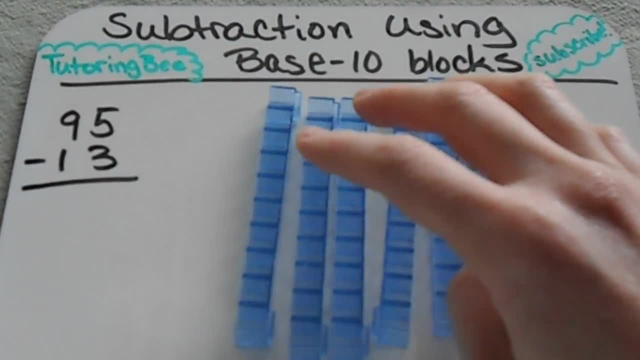 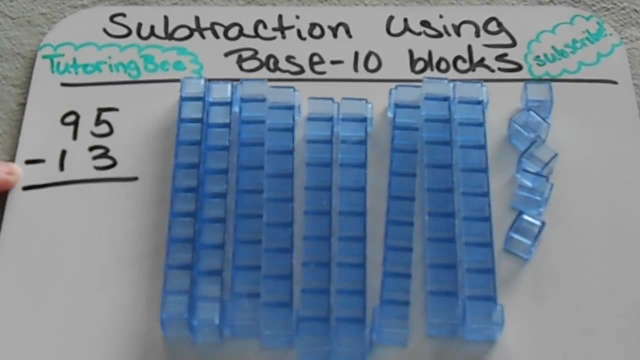 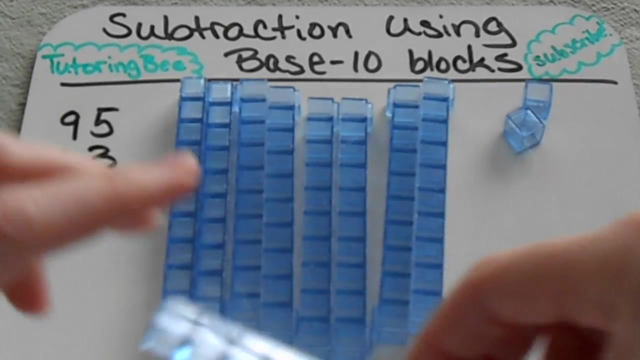 95, 1,, 2, 3, 4,, 5,, 6,, 7,, 8, 9.. So I've got my first number set up And then, since subtraction means take away, that's exactly what I'm going to do. I'm going to take away the. I'm going to start with my smaller place value, the ones place. I'm going to take away 3 of these ones, put those off to the side. I'm going to take away 1 of these tens, put that off to the side and then count up what I have left. I have 2 ones. 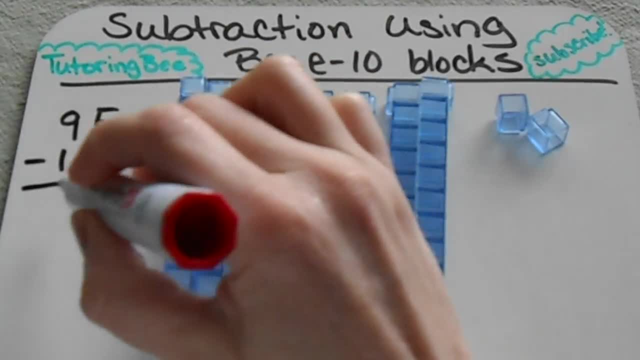 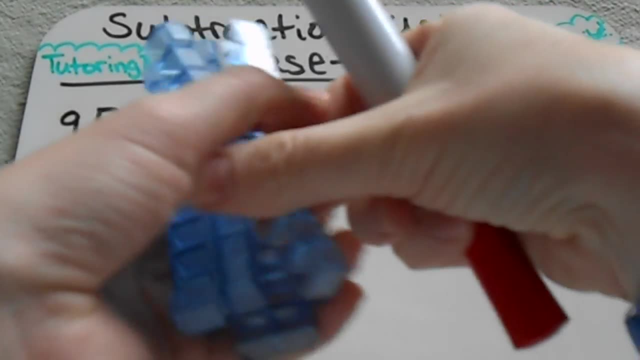 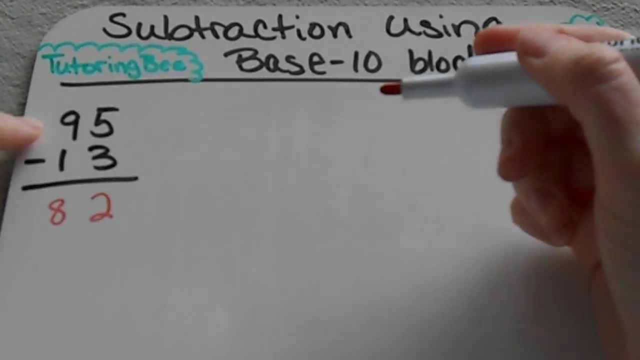 and 8 tens left, So my answer would be 82.. But again, I'm going to show you how you can solve this problem: by just using a pencil and paper, and you don't have to have the manipulatives. So I'm going to set up. 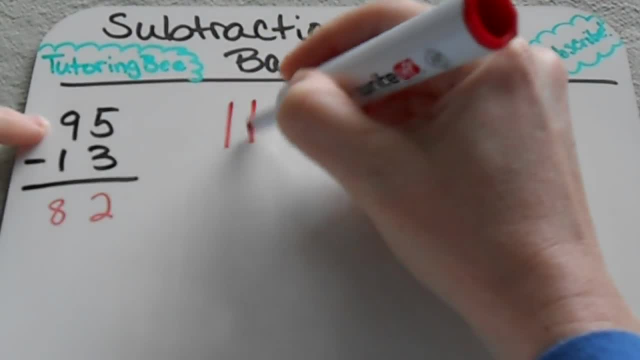 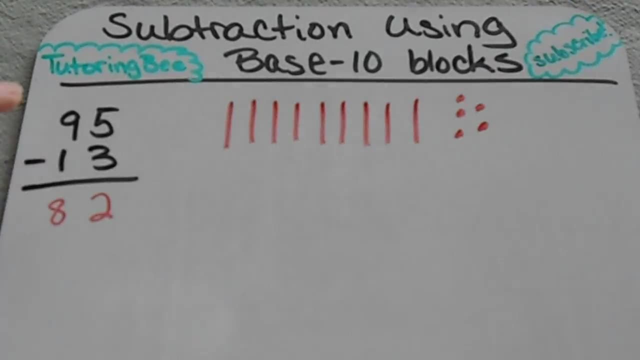 my problem the same way with 9 tens: 1,, 2,, 3,, 4,, 5,, 6,, 7,, 8,, 9, and 5 ones- And then, to show this on On paper, when you're subtracting, you actually just cross off three of those ones and then 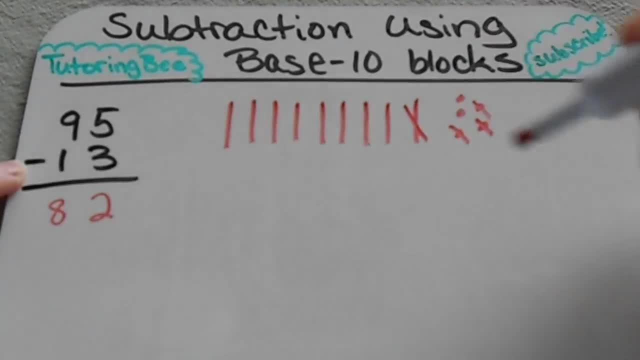 you cross off one of those tens and then you count up what you have left over: One, two, two ones, and then one, two, three, four, five, six, seven, eight, eight tens. Now, that one did not require any regrouping, but this one does, down here. 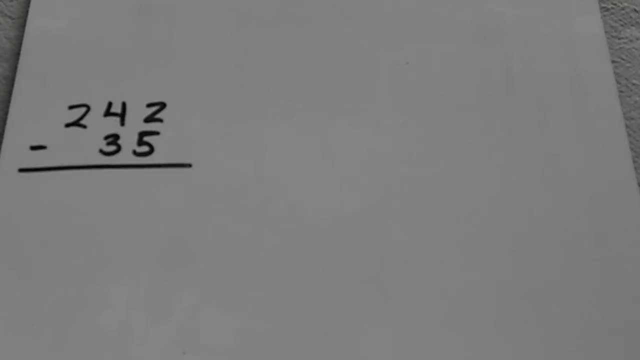 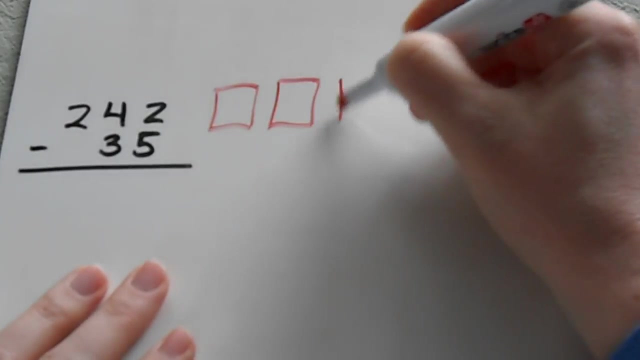 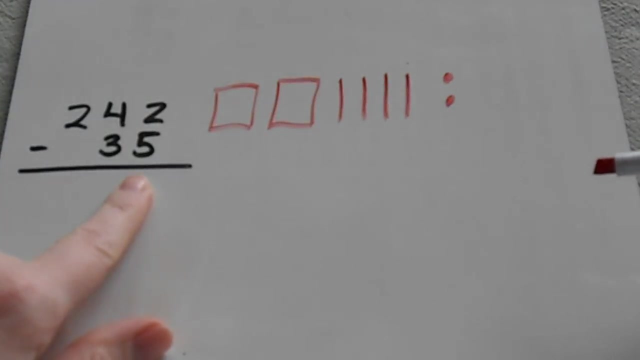 Again, I'm going to set up my top number with my base ten blocks. The hundreds uses these large flats, and then I need four tens and then I need two ones. So now we start subtracting. I always start with my smallest place value, the ones place, and then I subtract. however, 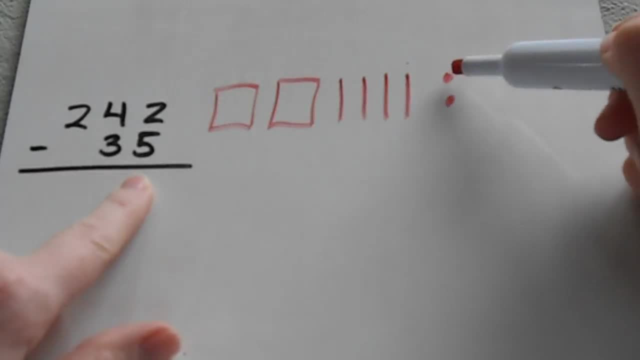 many ones I need. However, in this case, I do not have enough ones to subtract five of them. So where do I get more ones from? I go next door, I take away one of these, and one of these tens equals ten of these ones. 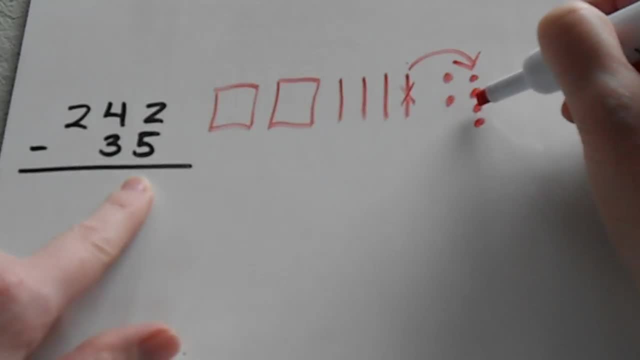 So I'm going to draw in another ten ones: One, two, three, four, five, six, seven, eight, nine, ten. Be careful with students that want to just make the whole ones place equal ten. So what I mean is, since there was already two here, they might say one, two and then. 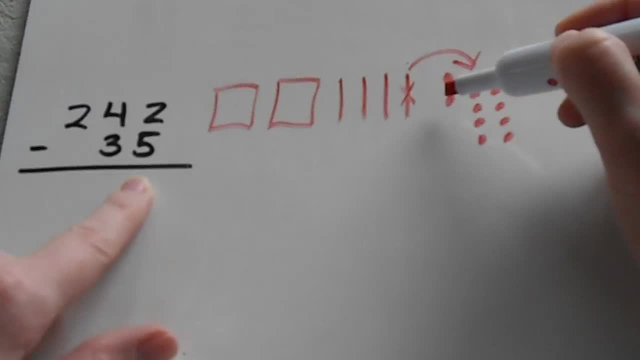 just add eight more to make ten total, But that's not really what they want. So what this means, This whole thing stands for ten. So no matter what you already have here, you're putting in ten more ones here, So now we have twelve ones. 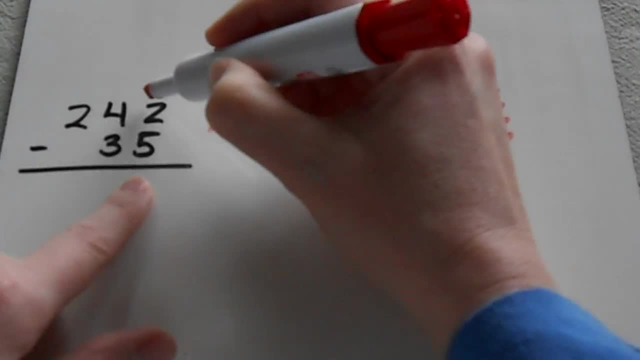 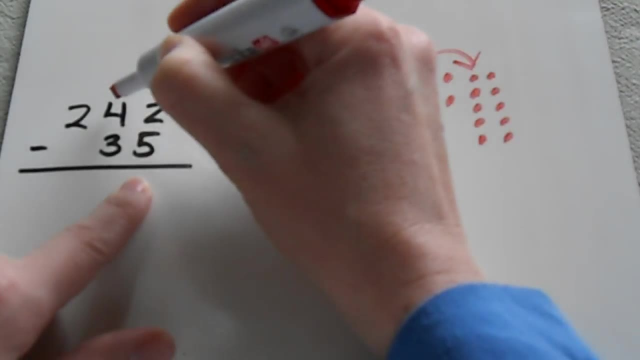 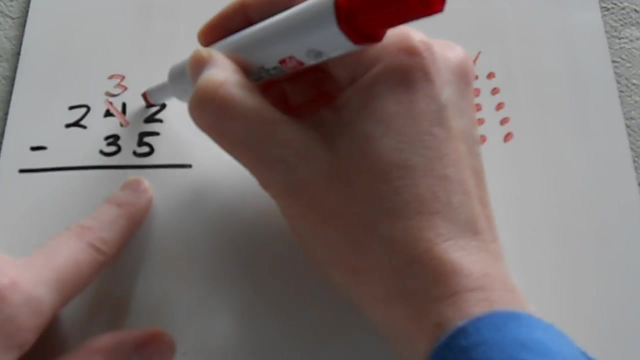 And you can actually start to show how to borrow or regroup on paper. So once you've done this step, show here what we just did. We took away one of these and now we have only three tens left, And instead of just two ones now we have twelve ones. 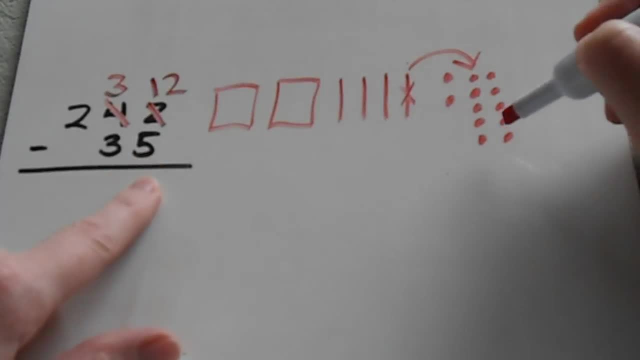 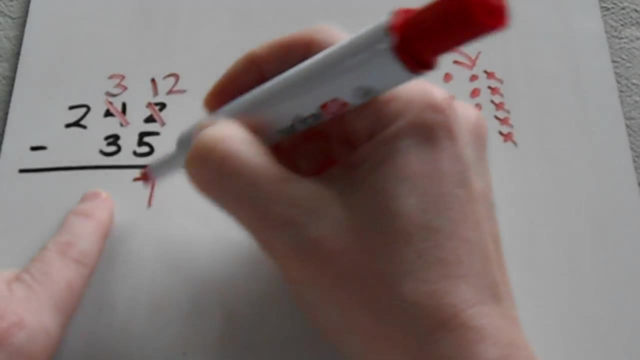 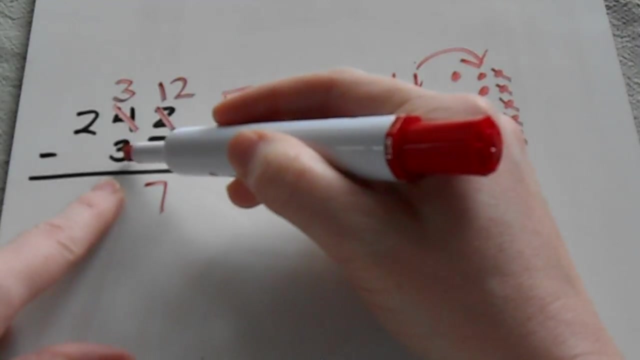 Okay. So now we can subtract five of these ones- One, two, three, four, five- and then count out what's left. I have seven ones left. Okay, now I move to my tens place. I can see that I'm taking away three tens. 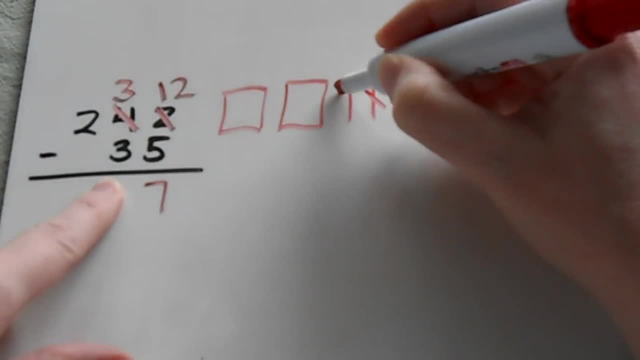 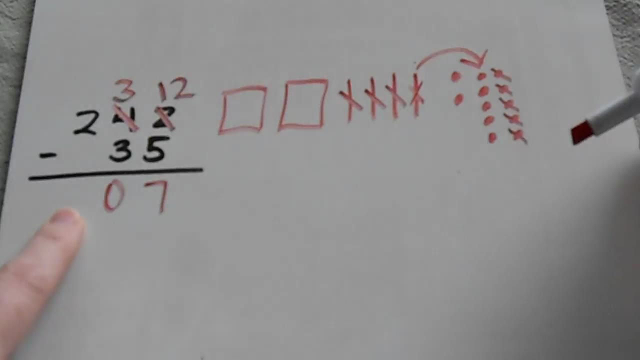 So I have enough to take them away: One, two, three, And since I already took this one out and gave it to the ones place, I have zero tens left And then nothing is happening, is being taken away from my hundreds place. 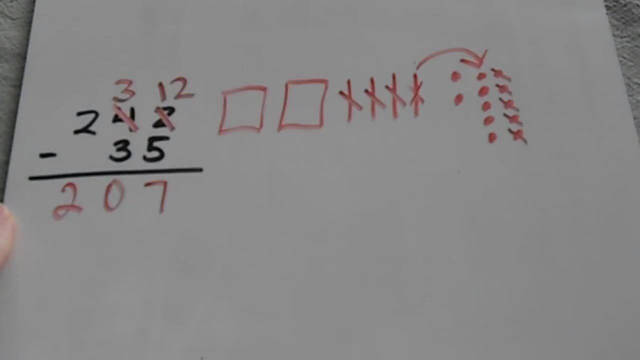 So I still have 200. So you end up with 207.. So that's just an easy way to visually see how the numbers are working together and how you're regrouping, And it's a great transition for students who are first learning how to regroup. 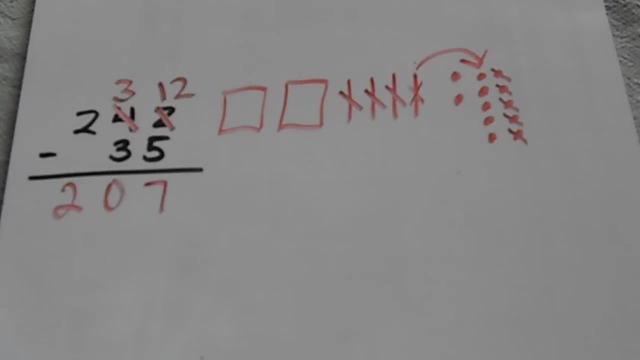 especially with subtraction, since it can be somewhat of a difficult concept. Thanks so much And I hope that you liked this video. Please subscribe to my other Tutoring Bay videos. Thank you.